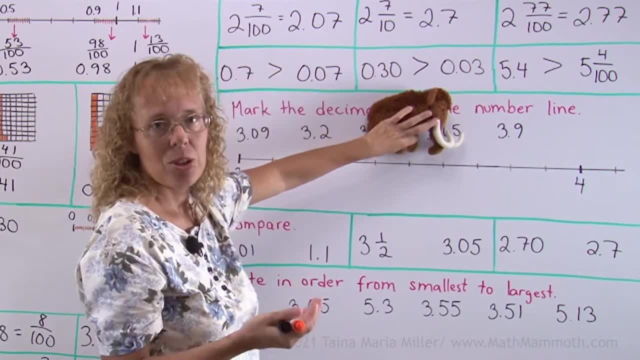 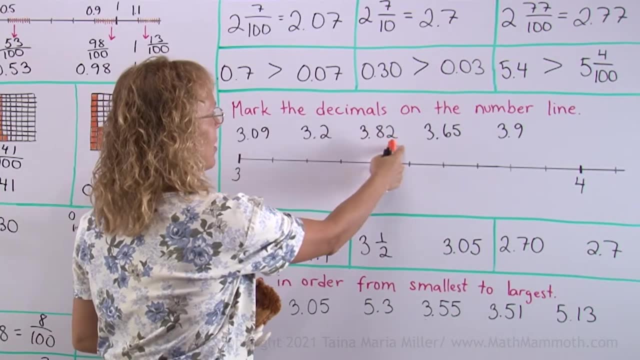 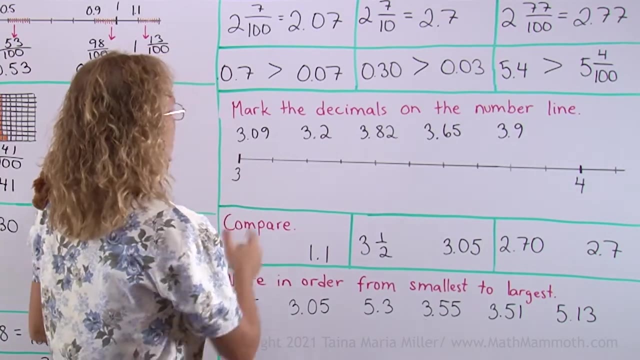 tenths to 3 and 5 tenths. So how much did he jump? He jumped 3 tenths. We could write an addition: 3.2 plus 3 tenths is 3.5.. Okay, thank you, Matthew. Enough jumping, now Let's. 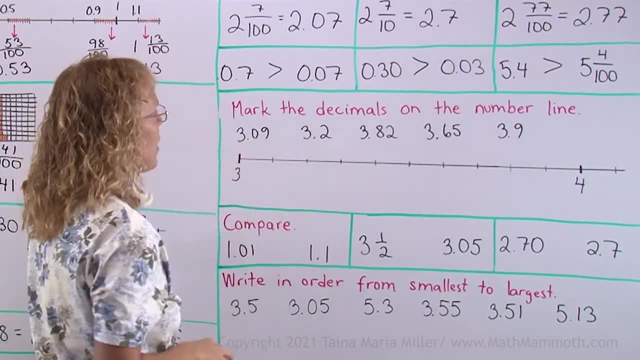 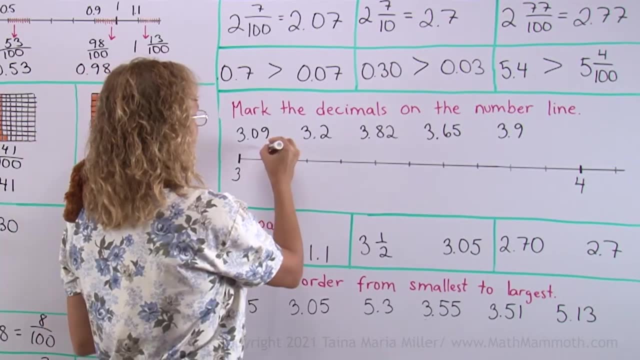 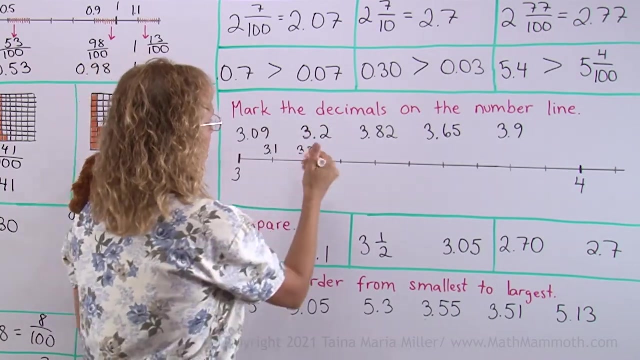 mark this on the number line 3.09.. 3.09.. Well, you see, the number line here is divided into tenths. So here I have 3.1.. Here I have 3.2.. Well, this is here 3.2.. Easy to mark because it's right there. It's this one here, Okay. 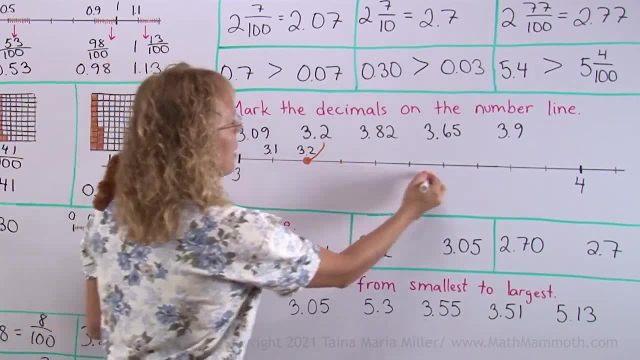 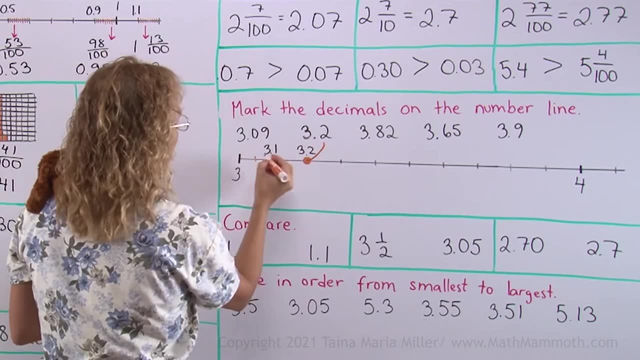 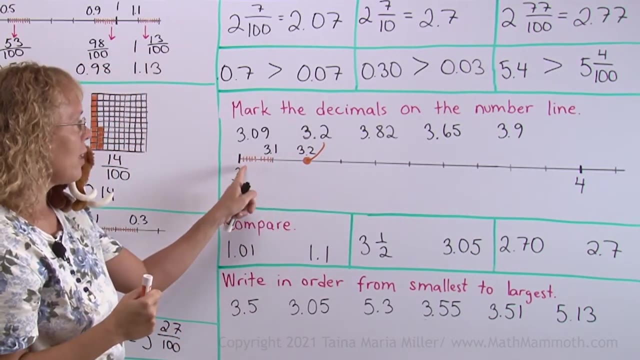 But where is 3.09?? Because none of these tick marks will be that. We need to now imagine that if this was divided into 10 little parts, just like I had there 3.09.. 3.09.. Okay, Didn't go evenly, Anyway. Then here would be 3.01.. And 3.09- is this one The tick? 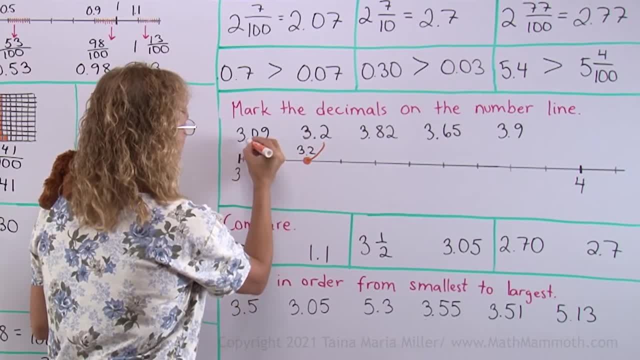 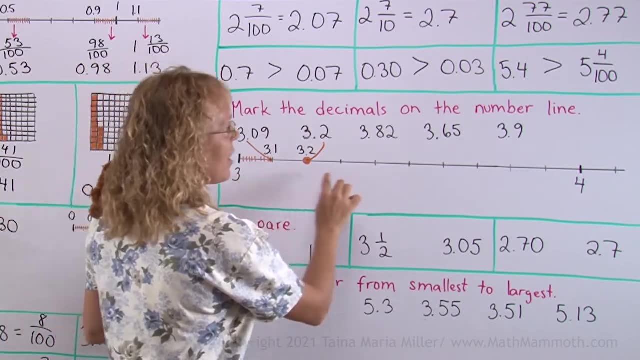 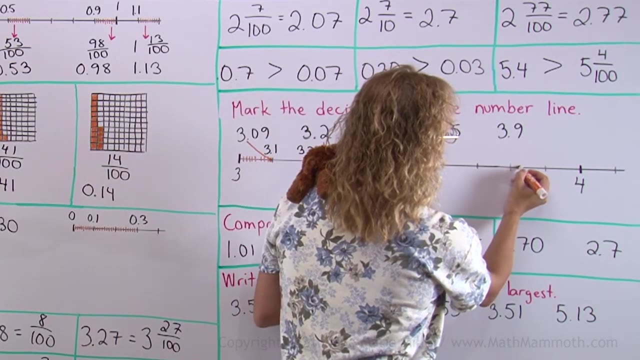 mark just before 3.1. Over here is 3.09.. 3.82.. I will first go to 3.8.. Or 3 and 8 tenths over here And then two hundredths beyond that. So two little thingies beyond that Somewhere. 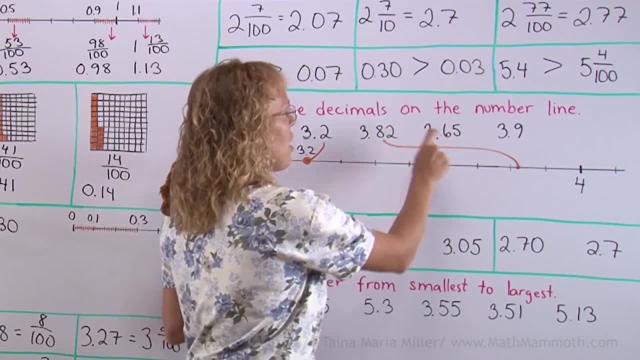 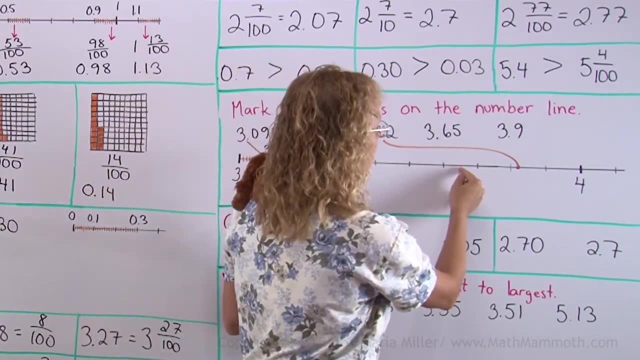 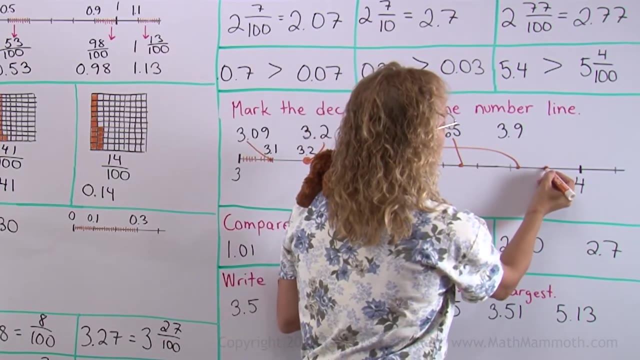 there 3.65.. 3.65.. First go to 3.6.. 3 and 6 tenths here And then go five hundredths more. It will be exactly in the midpoint here. And then lastly 3.9.. Well, that is easy. It is exactly the tick mark here for 3 and 9 tenths. 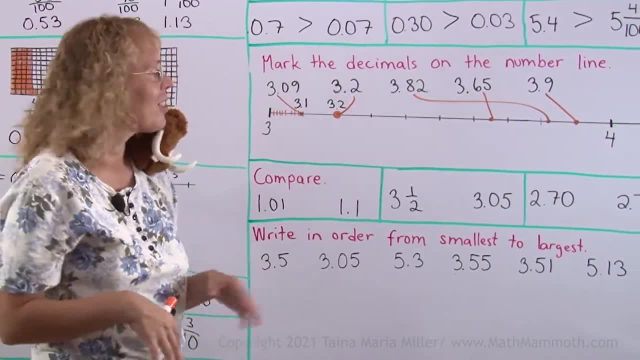 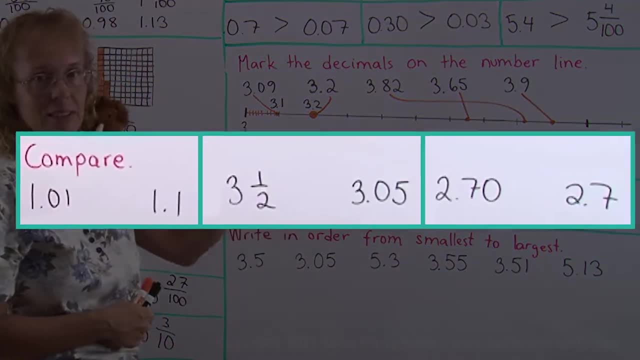 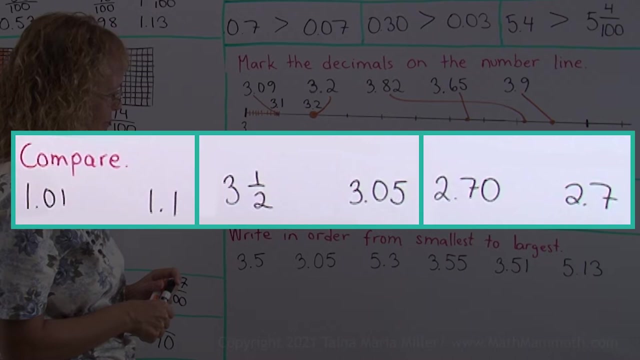 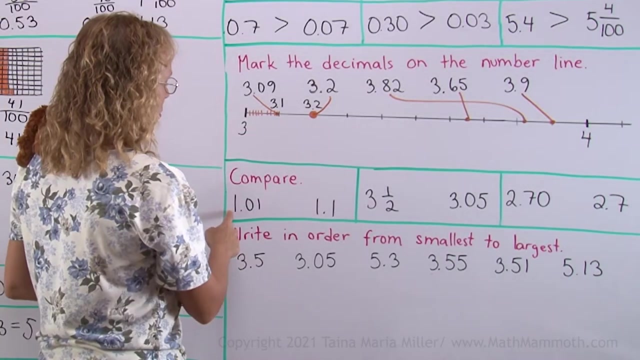 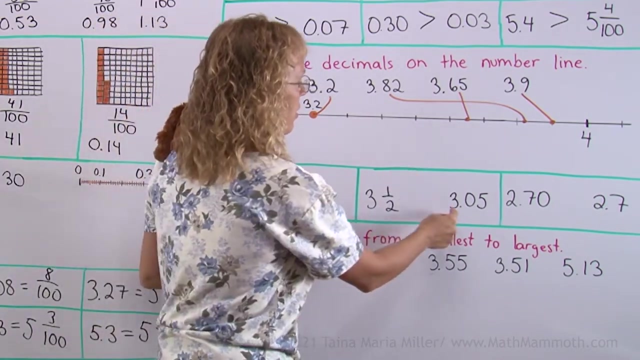 Compare again Now. if you're a student, pause the video now and try to compare on your own and see if you have understood these things in the lesson And if you can compare. Okay, Which number is greater? I have 1 and one hundredth. 1 and one tenth. 1 and one tenth is more. 3 and a half 3 and